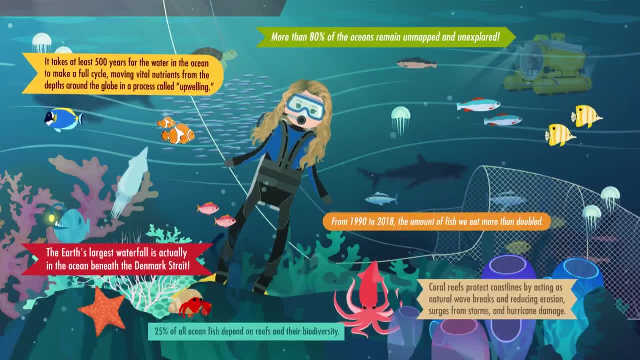 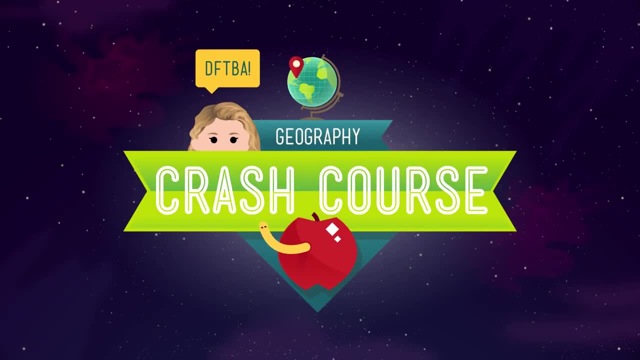 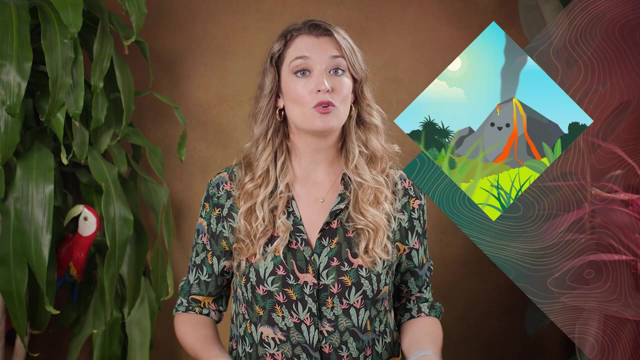 I'm Alizé Carrère and this is Crash Course Geography. Natural events are all the ways our restless Earth is constantly reshaping and modifying itself, Like volcanoes erupting or tropical cyclones… cycloning, And so far in this course, we've seen a lot of natural disasters. 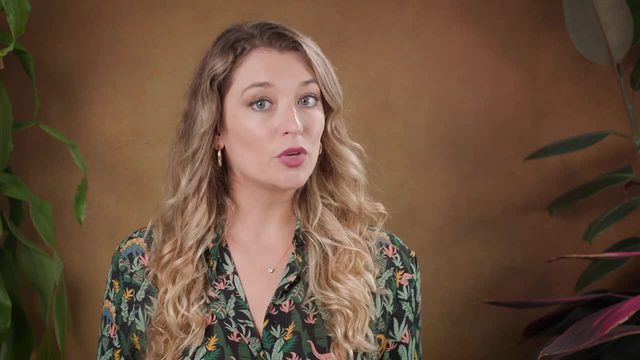 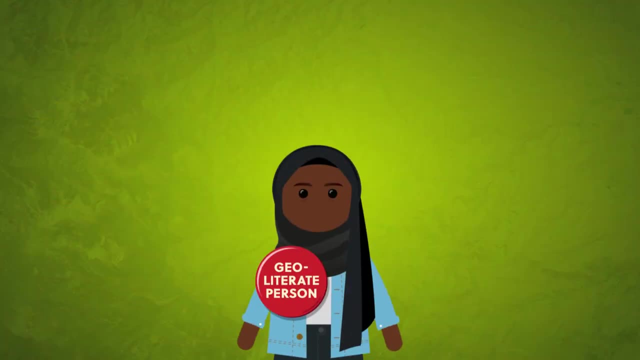 we've studied why these natural events happen, Like how it's really tectonic plates colliding and diverging that create the pattern of volcanoes along the Pacific Ring of Fire and many of those eruptions, But to be geoliterate people and fully understand what turns a natural event into a natural hazard, 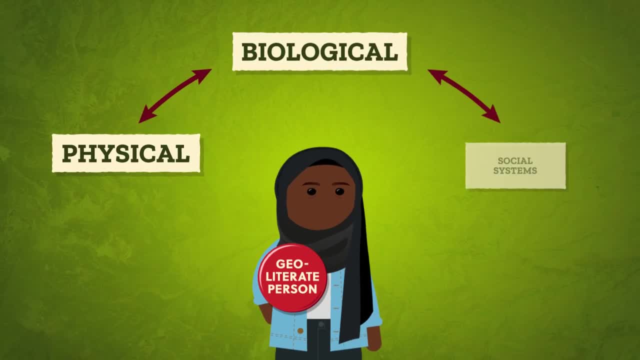 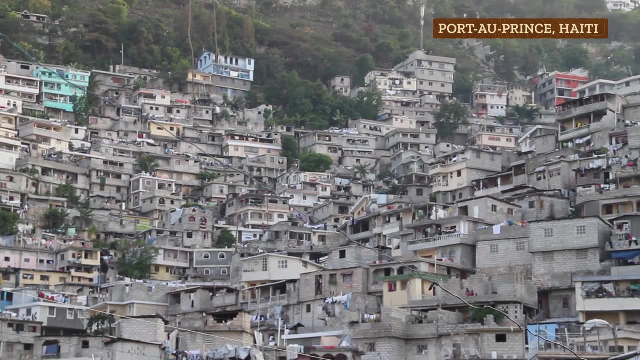 we have to remember that the world works as a set of physical, biological and social systems. So we also need to study things like how humans settle the land and how patterns of affluence, economics and politics contribute to disasters. The human geography stuff, In fact, every natural. 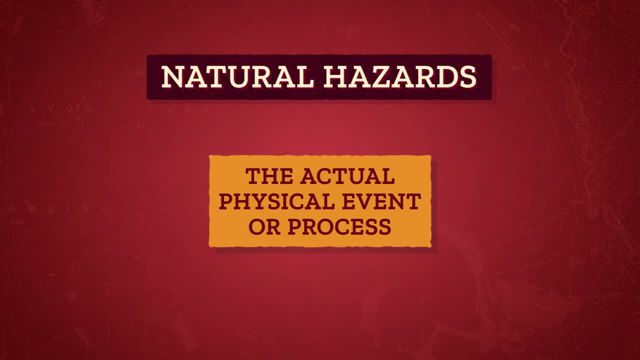 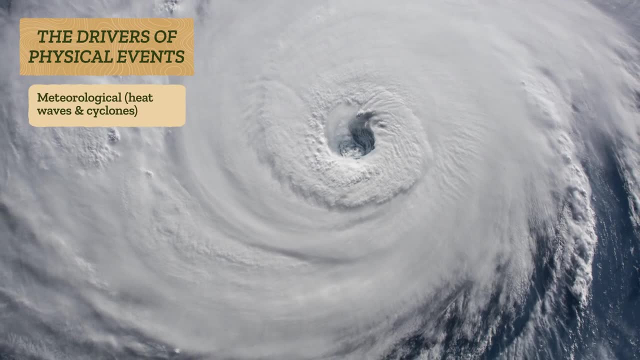 hazard has two main components: The actual physical event or process and the potential impact on humans. The physical events are driven by all the physical processes we've learned about. They could be meteorological events like heatwaves and cyclones, geological events like earthquakes. 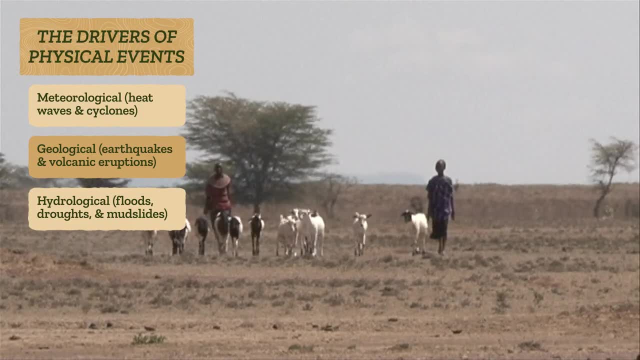 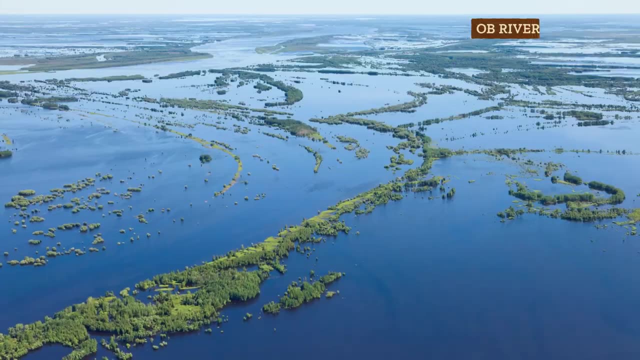 and volcanic eruptions and hydrological events like floods, droughts and mudslides. It's the second component, the impact on humans that changes a natural event into a natural hazard, Like severe flooding out where no one lives, like in parts of Siberia, is a much less severe threat. 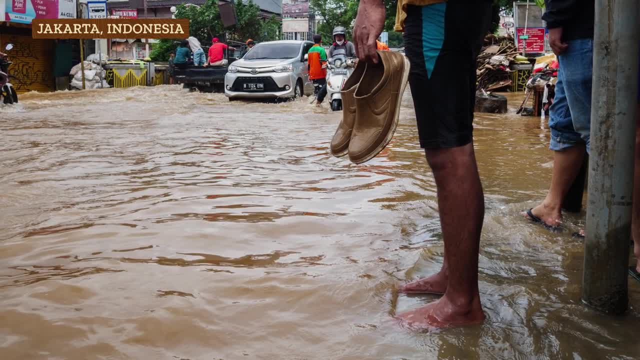 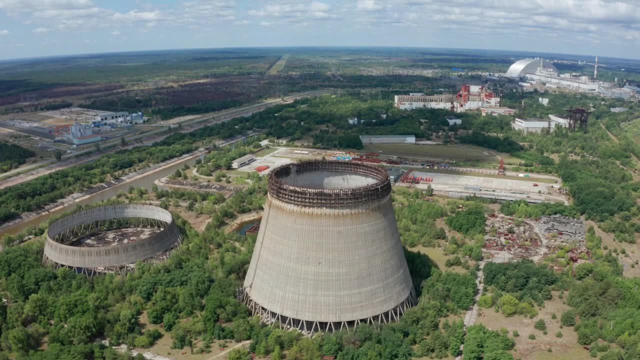 to humans, So less of a hazard than a mild flood in a densely packed city like Jakarta. But it's also important to clarify what a natural hazard is, not Something that's human-caused, like pollution, events like radioactive waste or oil spills. 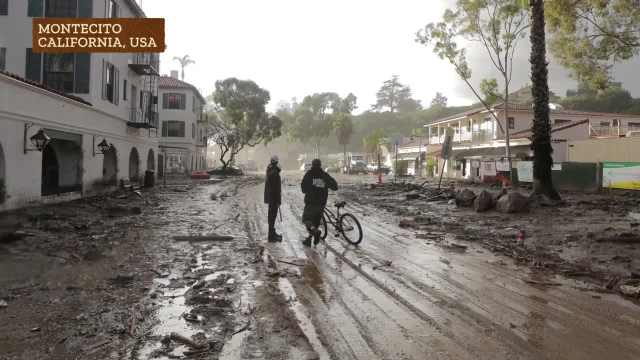 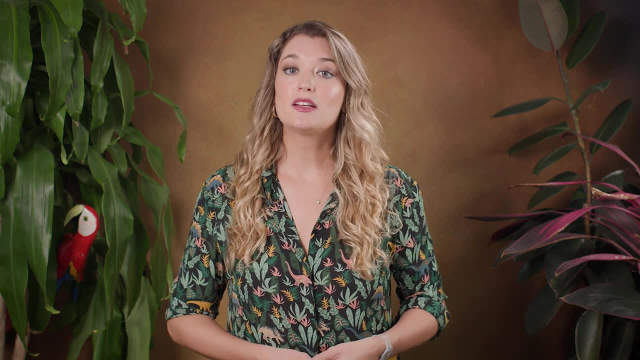 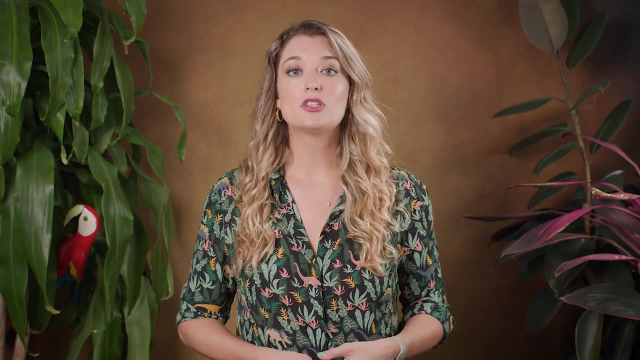 are considered human-made disasters and are normally excluded, And when the natural event actually happens and causes significant harm to humans, we call that a natural disaster. As geographers, we want to compare different places and answer: why would this hazard happen here and not there? So, in order to evaluate a hazard, geographers 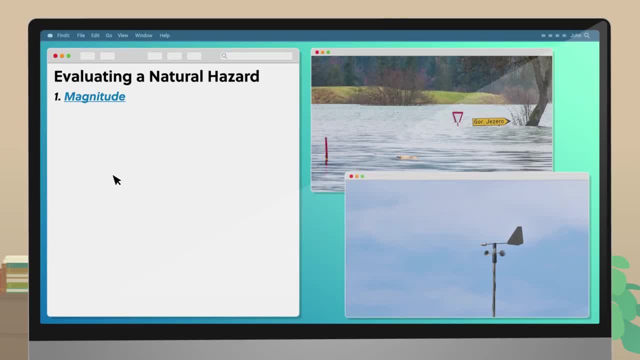 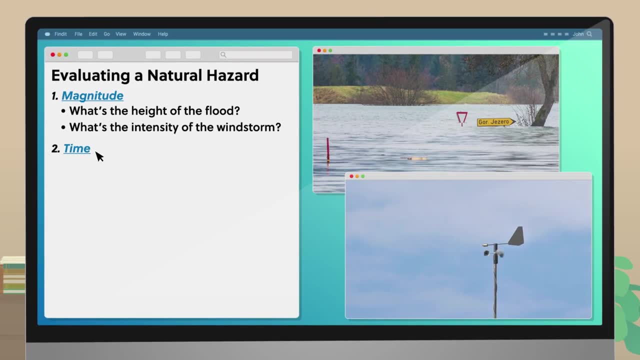 might look at several different dimensions, Like we might want to know how big the event was. in some way The height of a flood or the intensity of a windstorm measures the magnitude of the event. Time is also an important dimension to a hazard in many ways. 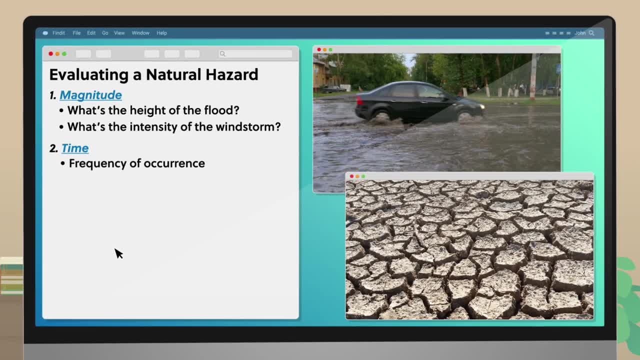 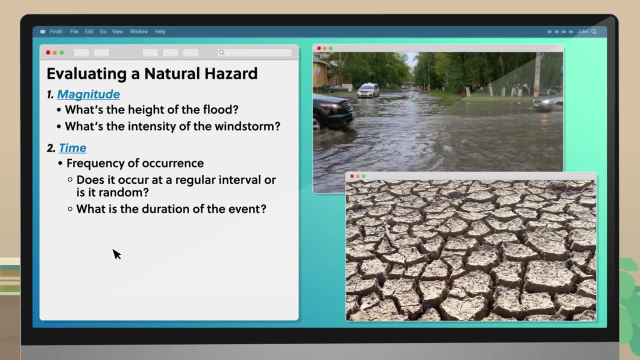 We might want to know about the frequency of occurrence, like if flooding is seasonal or rare, and whether it occurs at a regular interval or is random, and how long it lasts, or the duration of the event, And a drought might be weeks or months in the making, whereas a 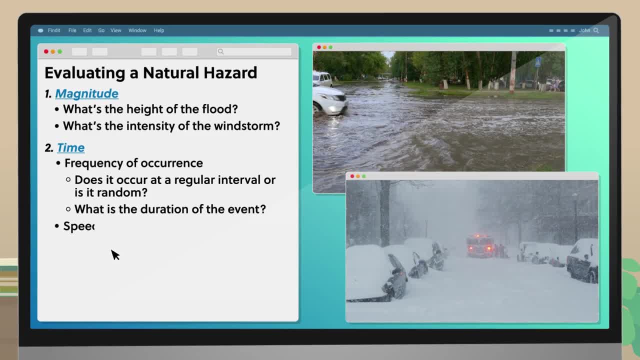 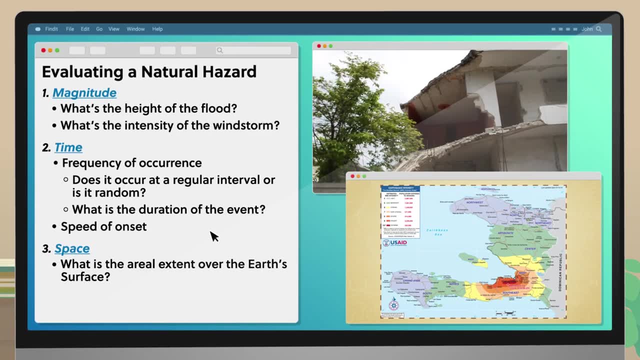 hurricane or blizzard can appear suddenly, So we can also look at the speed of onset. Of course, it's also important to look at the magnitude of the event, Like we might want to know how big an area was affected by an earthquake and the degree of spatial concentration within that. 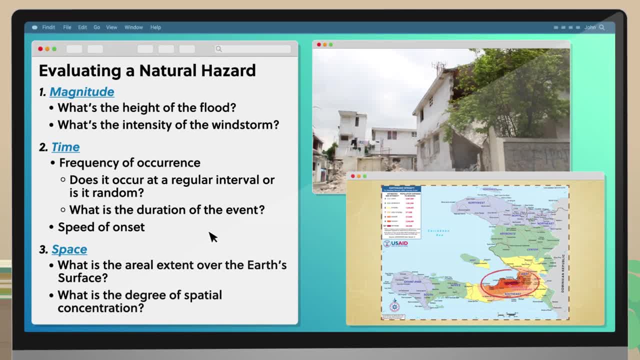 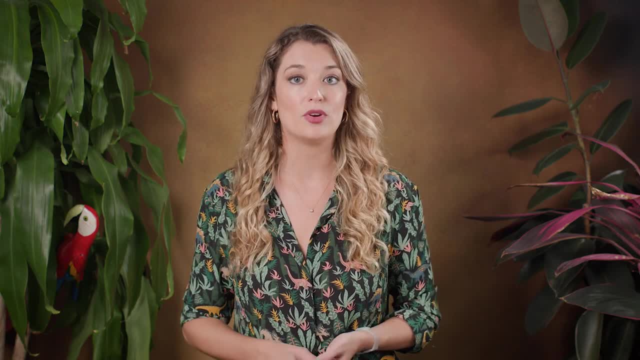 area Like the most severely affected area would be at the epicenter, where there were the strongest shocks. Evaluating hazards can also tell us how they've changed over time and show how the environmental and human components have become even more tightly intertwined As the human population has grown, we've tended to move into areas that are very attractive. 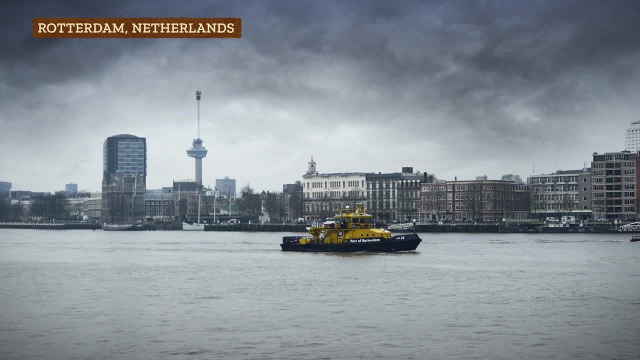 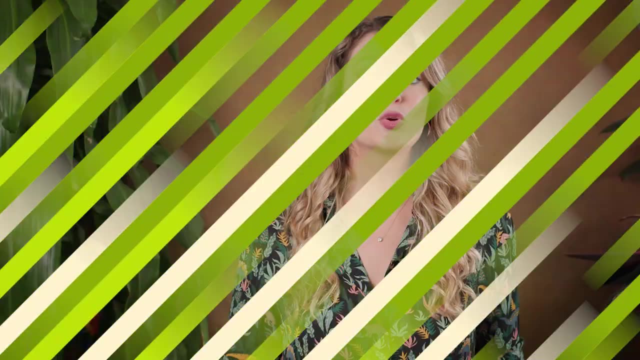 but also pose a high level of environmental danger, Like many cities are located in coastal areas. Or there could be other advantages, like rich volcanic soils that enable banana plantations. Our choices and social systems are increasing the impact of natural events and making some 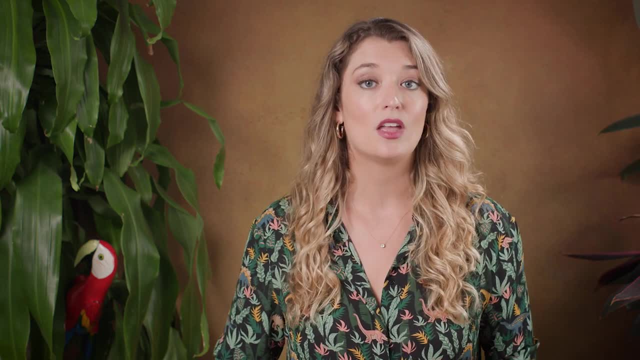 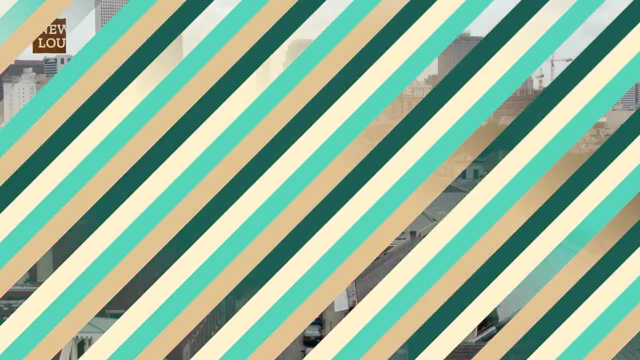 people and places more vulnerable to certain types of hazards than others. Where we can find opportunities or what we can afford money-wise has a big influence on what we're willing to accept risk-wise. Like in the American South, about half of New Orleans currently sits below sea level. 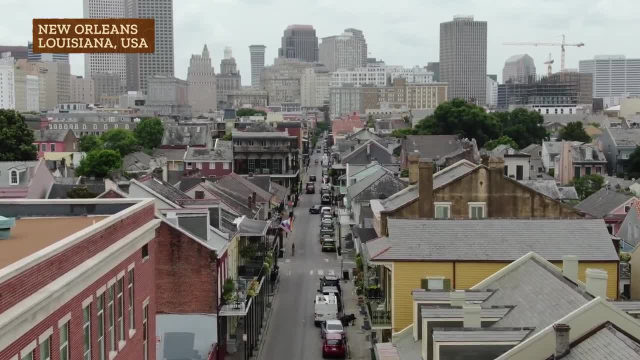 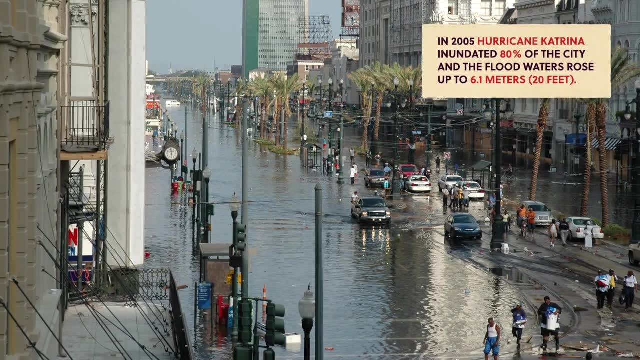 and people with low incomes live in the lowest-lying areas, making them more vulnerable to flooding, And when, in 2005, Hurricane Katrina inundated 80% of the city and the floodwaters rose up to 6.1 meters, these people were hit hardest by disaster preparedness and response. 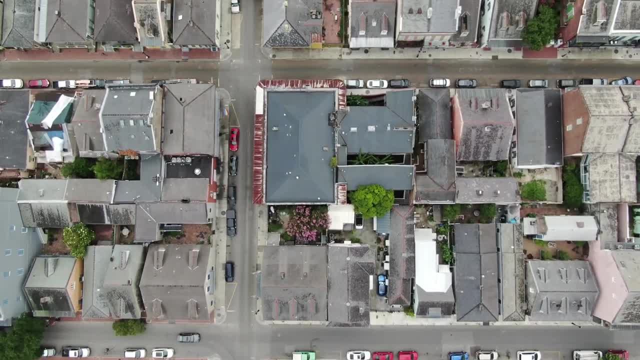 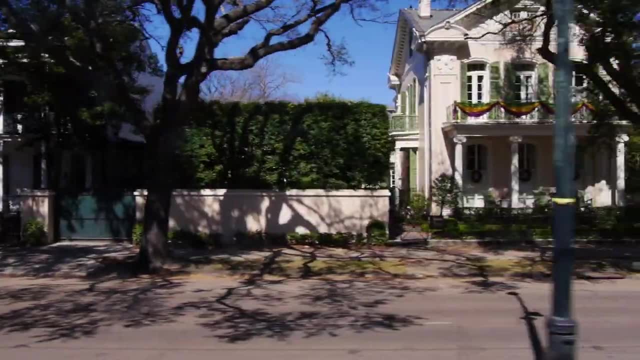 problems, But a poor response during a single disaster isn't the whole story. The tax base in New Orleans was eroded because of white flight in the 1950s, 60s and 70s, when white people who were usually better off financially or were able to participate in banking and real estate. 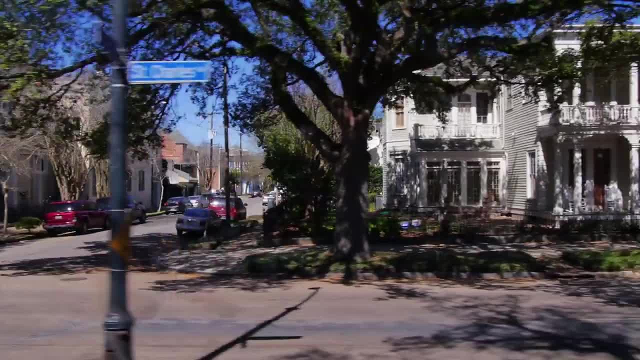 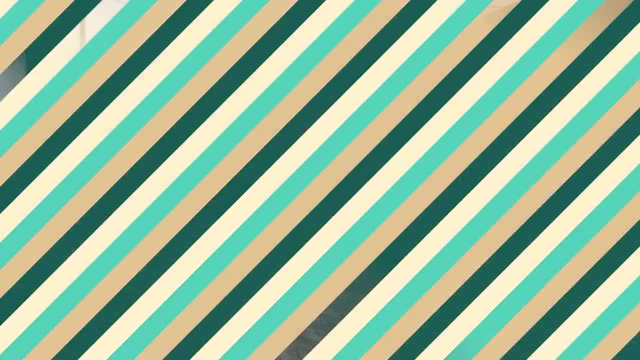 markets, relocated en masse from the central city to the suburbs. The people left had, all together, less money that could be taxed, so over time there wasn't enough investment in the city's drainage infrastructure. Because of more situations like Hurricane Katrina, many geographers now think 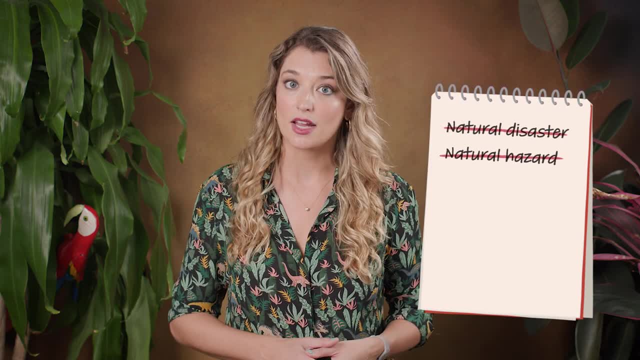 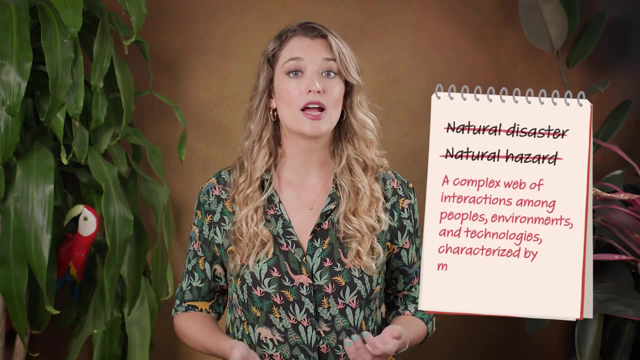 that phrases like natural disaster or natural hazard are misleading, And there's a push to define it as a complex web of interactions among peoples, environments and technologies, characterized by multiple causes and consequences, Which also means there's a lot that affects how vulnerable people are in a place. 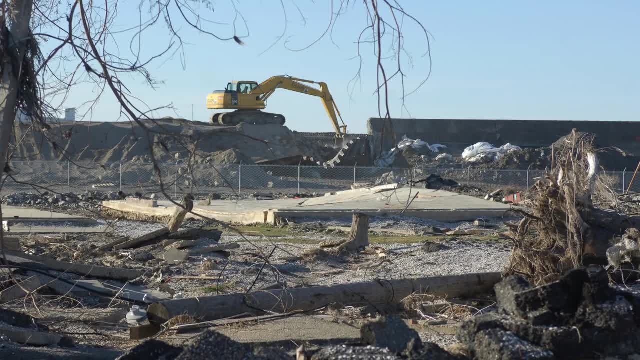 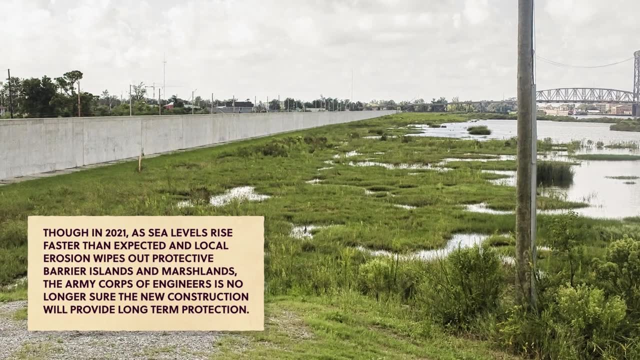 Like. it's generally understood that wealth, education, a high degree of social organization and advanced technology reduce vulnerability. As New Orleans rebuilt, a lot of energy and money was focused on strengthening levees, flood walls, floodgates and pumping stations to reduce vulnerability to future hurricanes. But as geographers, we want to. 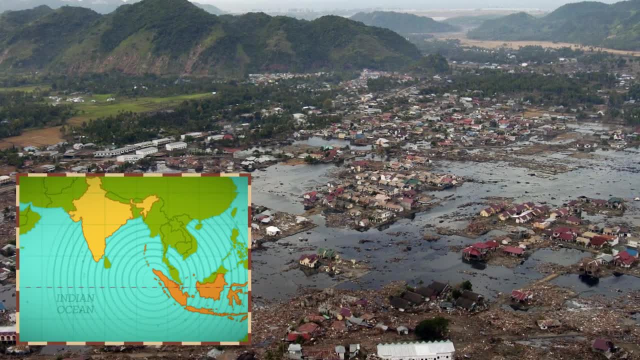 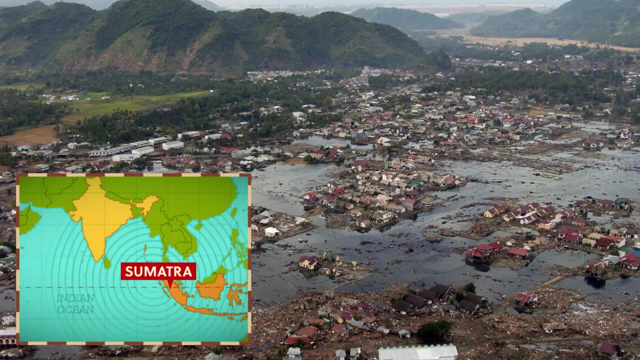 know if that's true everywhere. The Boxing Day Tsunami of 2004 along the northwest coast of what's now the Indonesian island of Sumatra was one of the most cataclysmic natural events of modern times. Its tremendous force and scope killed more than 230,000 people in 14 countries. 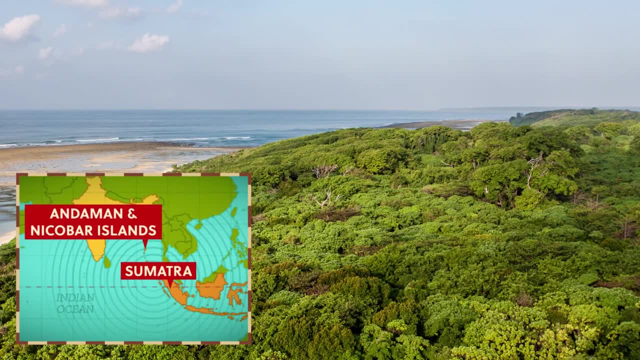 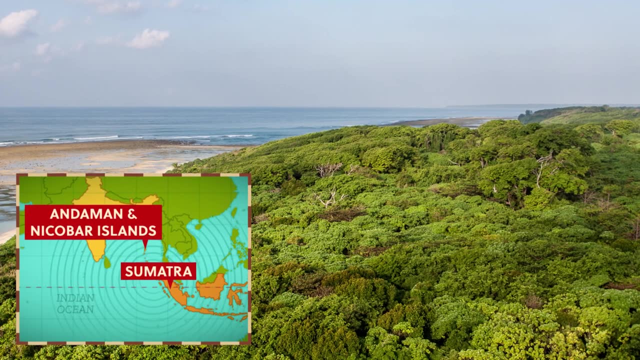 But in the Andaman and Nicobar Islands, a group of islands off the southeast coast of India, the Anj, a tribe of about 100 people, survived by taking shelter on higher ground, deep in their forest, to escape the fury of the wave. The Anj have lived on the island of Little Andaman for. 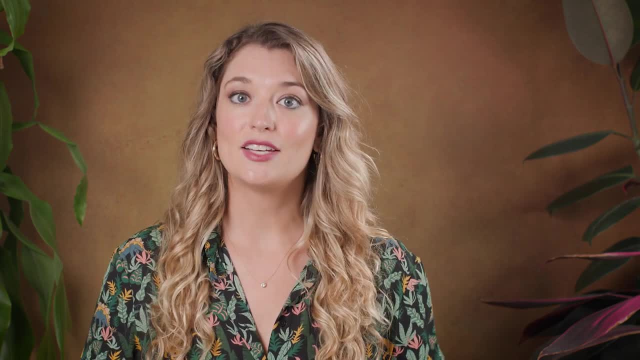 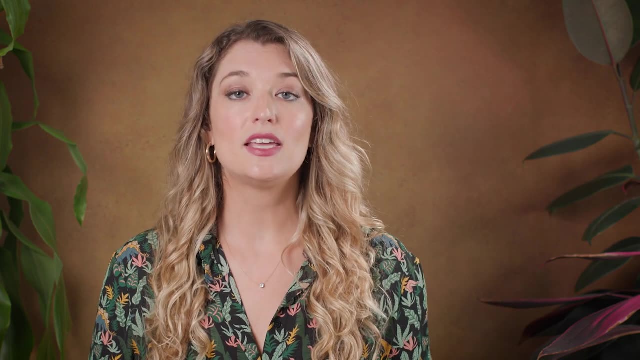 30,000 to 50,000 years. Their oral traditions had taught them about tsunamis and their folklore spoke of a huge shaking of ground followed by a high wall of water. They survived by heeding their traditions, though their settlements were completely destroyed. 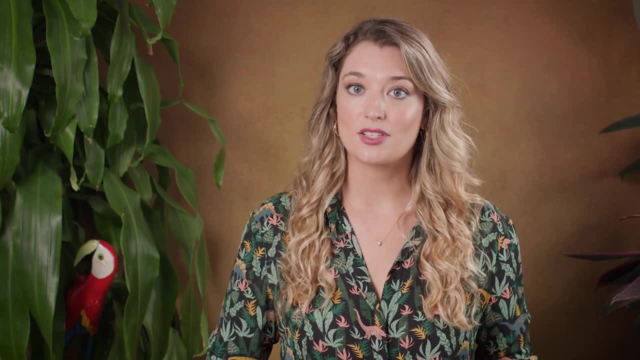 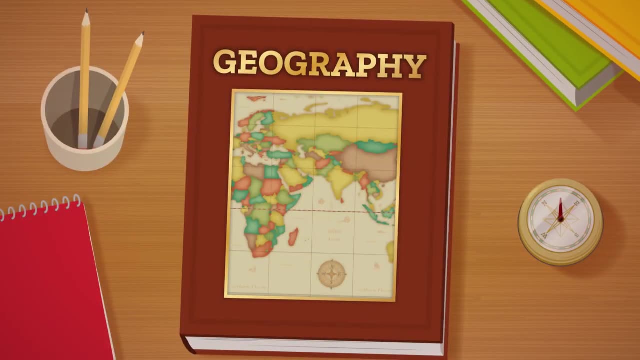 So, as we're assessing vulnerability and studying how to mitigate natural disasters, we have to consider all the ways different peoples relate to their environment and the value of different types of knowledge. Textbooks and classroom instruction are useful, but experience from keenly observing and living. 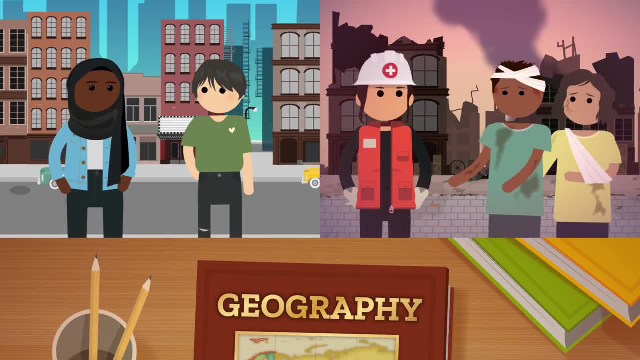 in the world is every bit as valuable, And this is why many geoliterate, geographers and disaster preparedness teams spend a lot of time in the field, talking with local residents of their communities and learning about this knowledge, Assessing how vulnerable a place is or was. 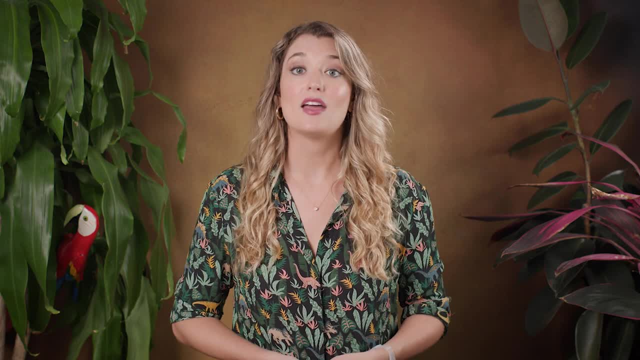 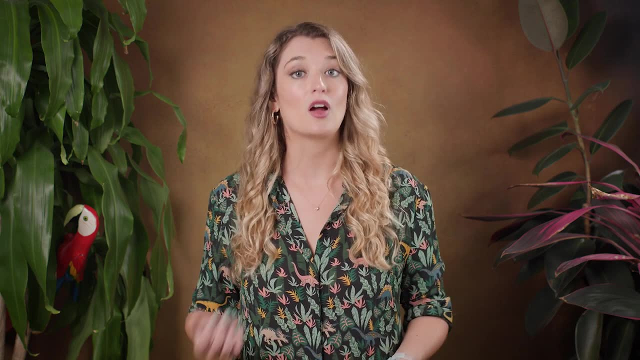 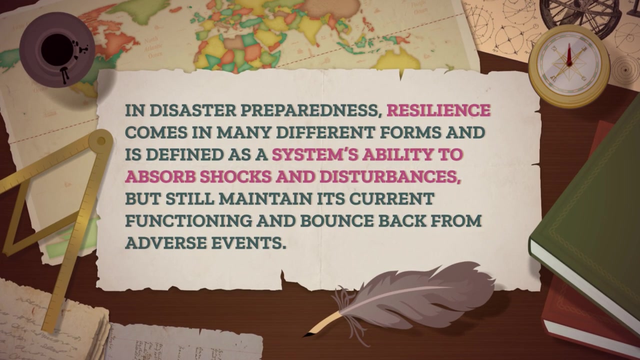 helps us learn a lot about natural hazards, but we also have to deal with the aftermath. The idea of resilience is an important aspect of disaster risk management because it shifts the focus from vulnerability to recovery In disaster preparedness. resilience comes in many different forms and is defined as a system's ability to absorb shocks and disturbances. 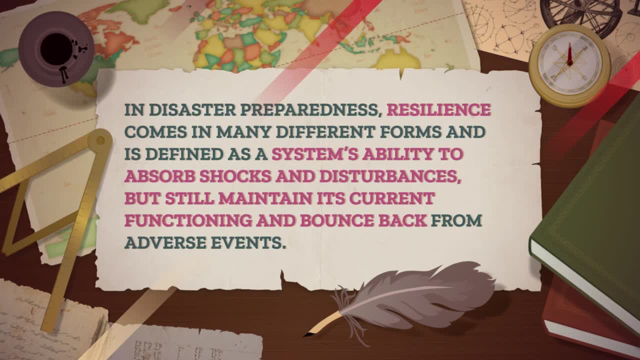 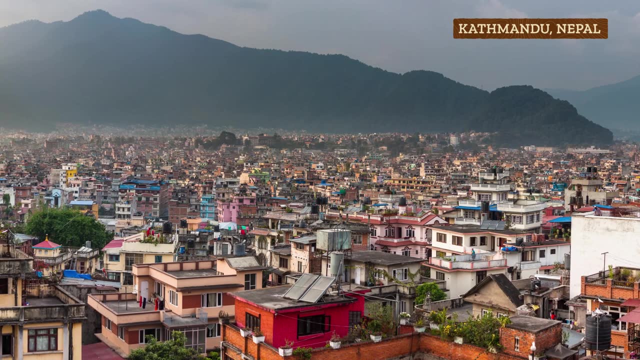 but still maintain its current functioning and bounce back from adverse events. For instance, traditional town planning and land use in the Kathmandu Valley has built a strong sense of community which fosters social resilience, which is when the social bonds of a community help it recover faster In older historic towns in Nepal. 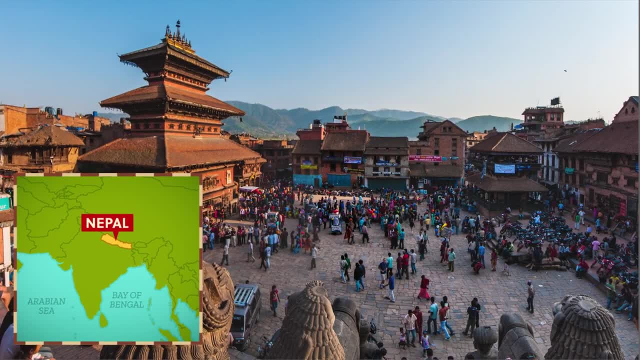 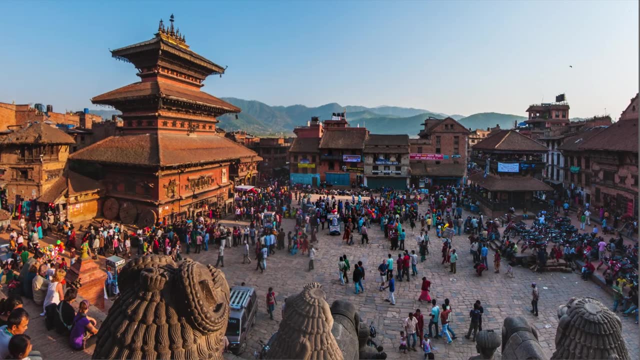 traditional open spaces like paved courtyards, chalks, neighborhood squares and larger open spaces at the edge of towns bring communities together during feasts, festivals and rituals, And during the Gorkha earthquake of 2015,, the community used these spaces as evacuation sites. 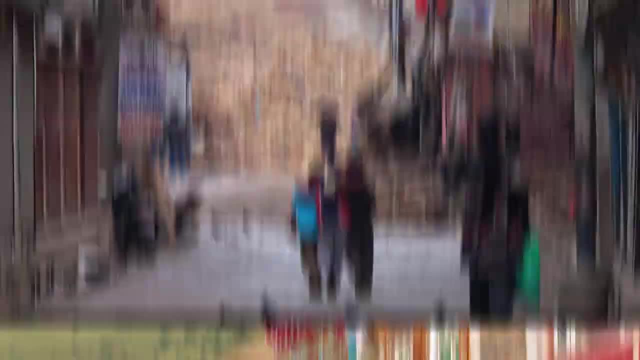 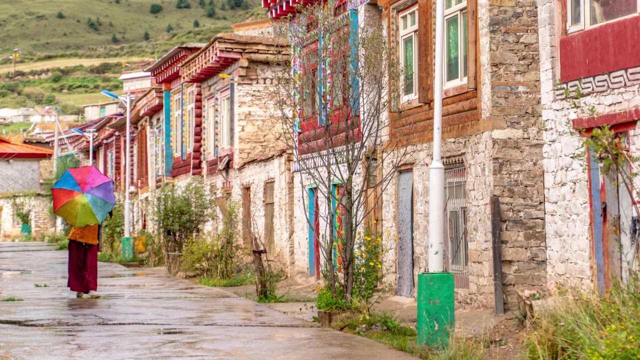 and to provide refuge for households during and after the disaster, And the architecture in these towns uses mixed timber and masonry construction and specifically represents the local culture and technology, but also functions as earthquake resilience. The buildings and houses are designed to absorb external forces and withstand displacement during an earthquake. 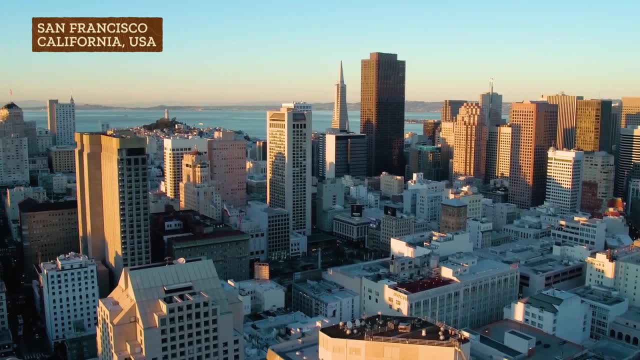 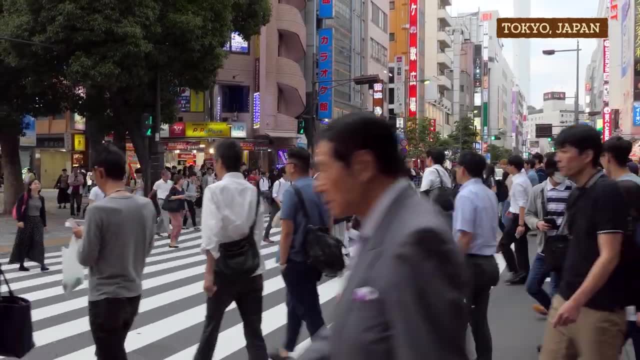 But this style of architecture wouldn't necessarily help the resilience of a city like San Francisco or Tokyo, where skyscrapers and high rises are common. Different cultures can have different attitudes about risk, the role of government and collective social responsibility too. Usually, what makes a place resilient locally or regionally is really specific. so there's no universal solution. But resilience implies a way forward, and enhancing the resilience of cities and communities is a broad policy objective at international, national and subnational levels. But no matter how prepared we are, some things can never be recovered after. 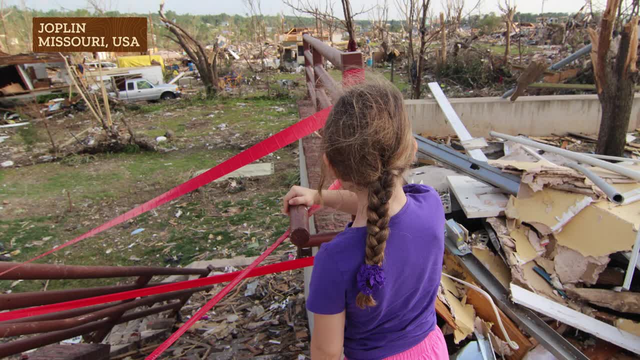 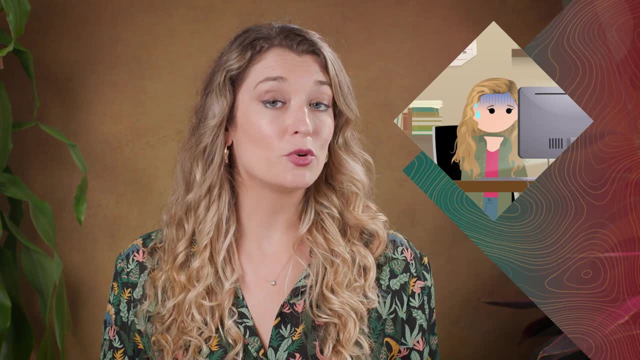 a natural disaster. Homes and businesses can be rebuilt and belongings can be recovered, but we've also lost a place and our sense of, and attachment to places. So there's a serious element to our where would you live game. Natural hazards constantly threatening our home is emotionally exhausting, but for some there's no other choice. 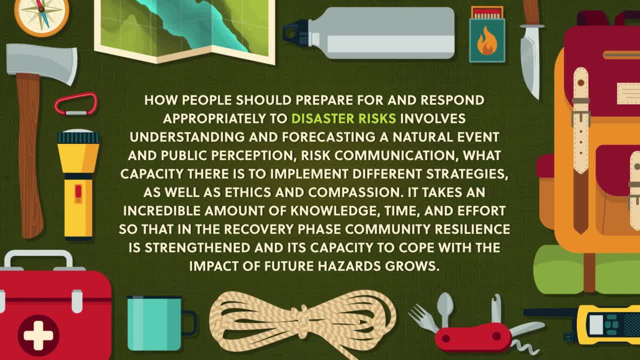 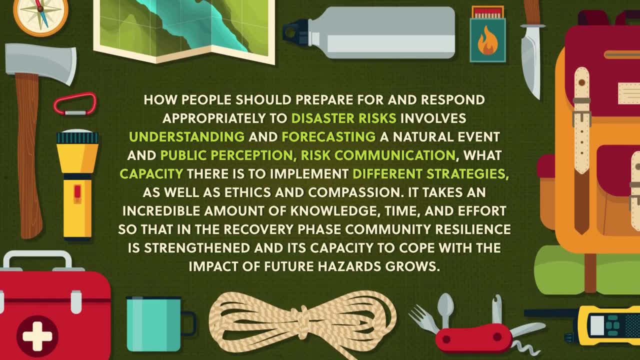 How people should prepare for and respond appropriately to disaster risks involves understanding and forecasting a natural event and public perception, risk communication, what capacity there is to implement different strategies, as well as ethics and compassion. It takes an incredible amount of knowledge, time and effort so that in the recovery phase, 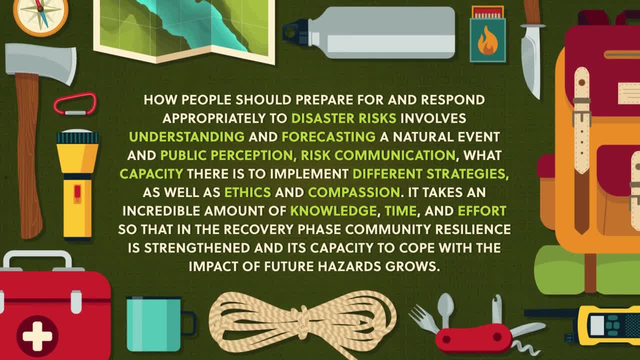 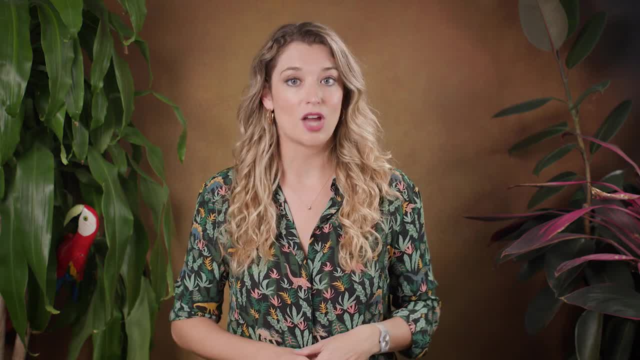 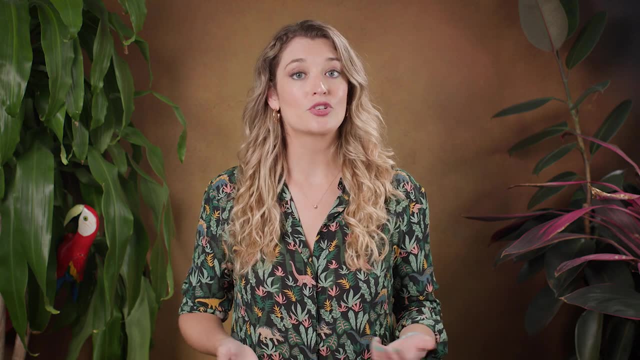 community resilience is strengthened and its capacity to cope with the impact of future hazards grows. Likely, no place is entirely safe from natural hazards, especially as social and environmental challenges multiply. But as we conclude the physical geography half of our series, we're hopefully better able to understand how rock structures, landforms, soils, vegetation, climate,